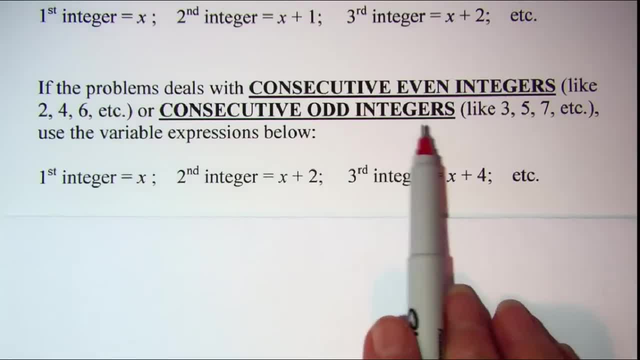 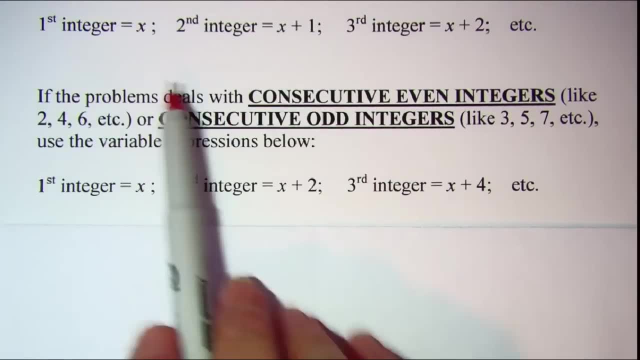 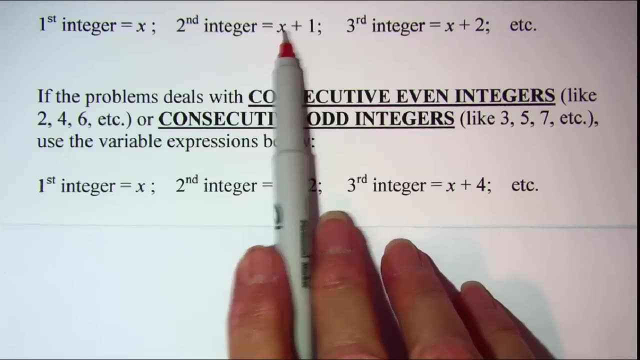 add 2 to get to the next one, and when you have odd integers as well, add 2 to get to the next one. So, either way, always let x be your first integer and then, if you're just dealing with consecutive integers, you'll go x plus 1, x plus 2, x plus 3, and so forth. 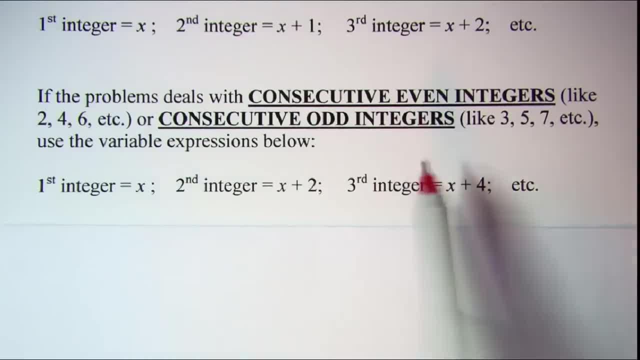 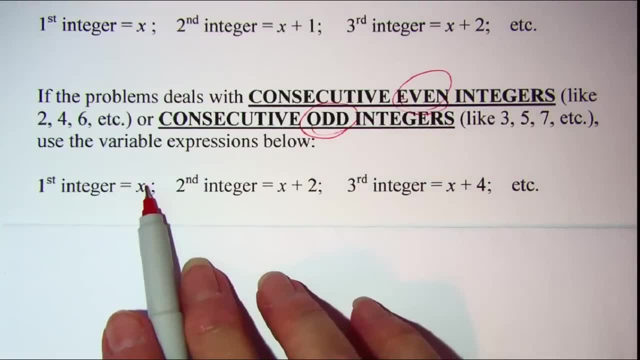 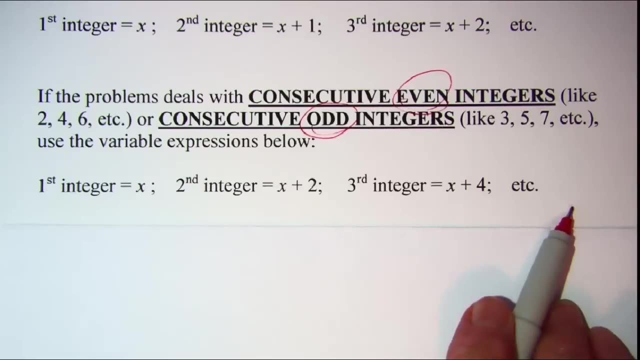 If you're dealing with either consecutive even or consecutive odd- either one of those- then you'll start with x as your first integer, and then x plus 2, x plus 4, x plus 6.. So let's do a problem. 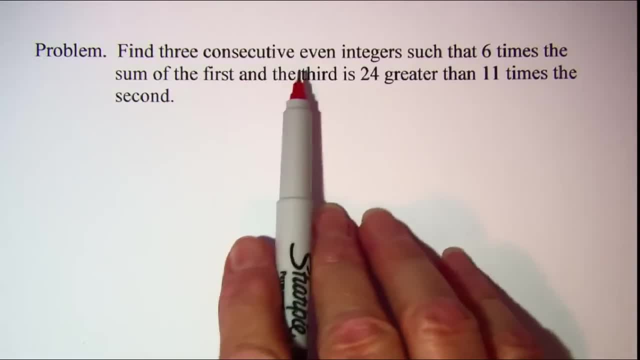 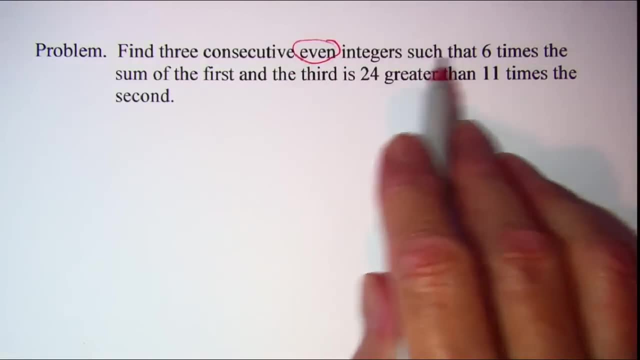 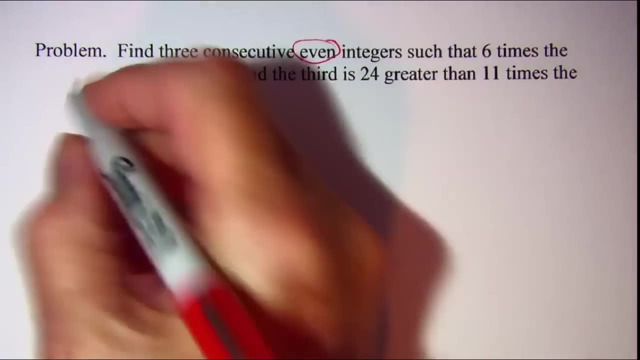 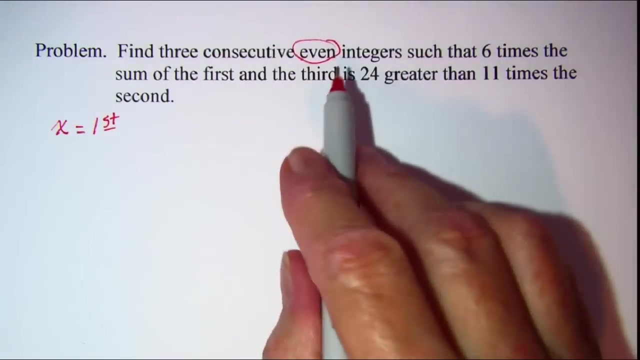 Our problem is to find three consecutive even integers, Even integers Such that 6 times the sum of the first and the third is 24 greater than 11 times the second. So always let x be your first integer and then, since I'm going with even integers, that: 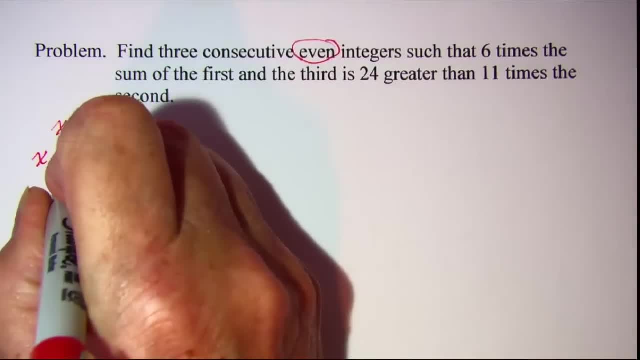 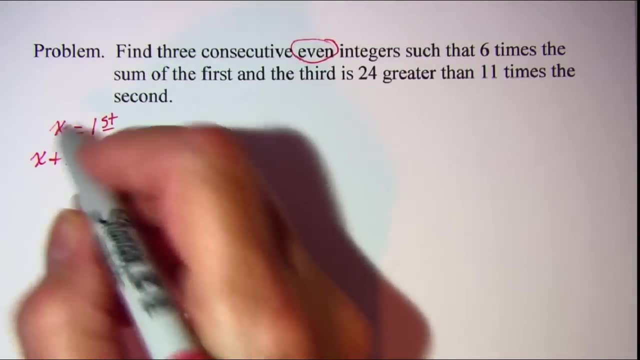 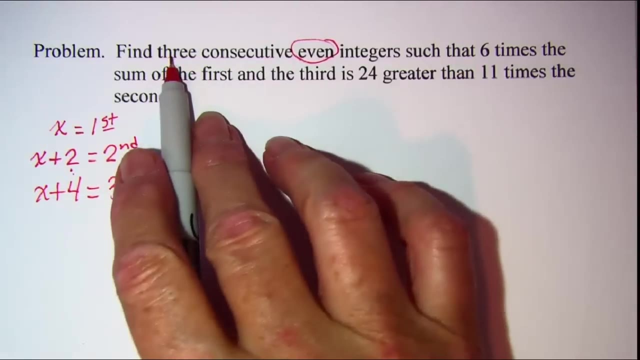 means that I need to use x plus 2 as my second and then skip over the next one. so add 2 onto this be x plus 4.. So I'm going to use x plus 2,, x plus 3, x plus 4, will be my third, and all I want is three. 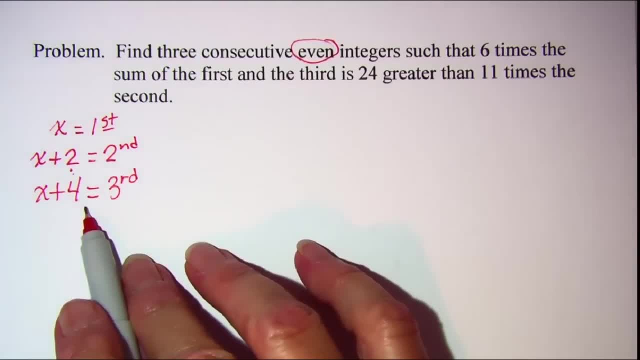 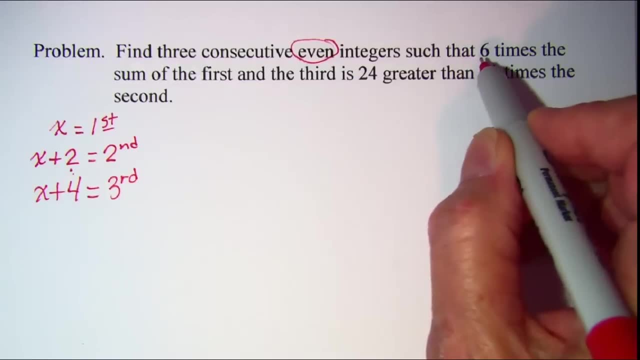 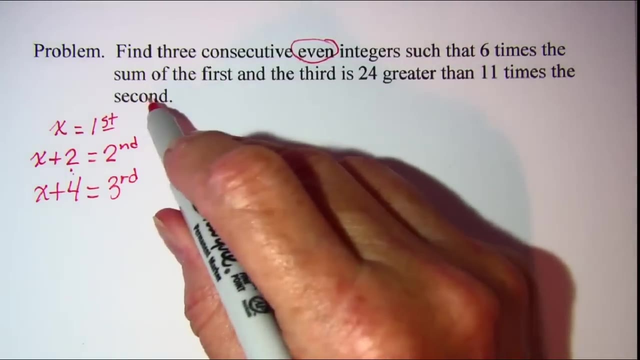 integers. so this should be fine for the translation of our problem. Alright, so now I'm going to start right here and start translating. So I need 6 times the sum. So I have 6 times the sum. So I need 6 times the sum. 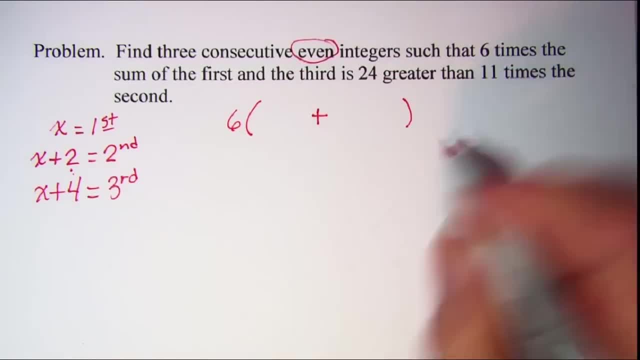 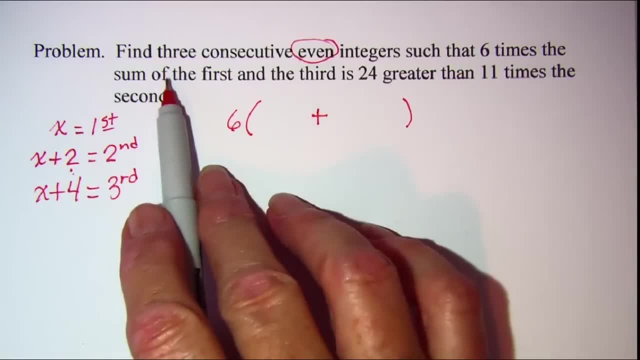 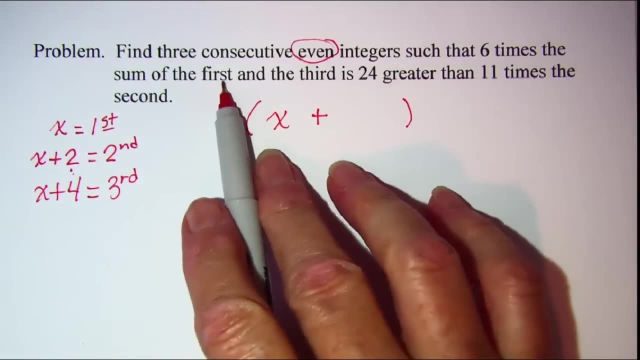 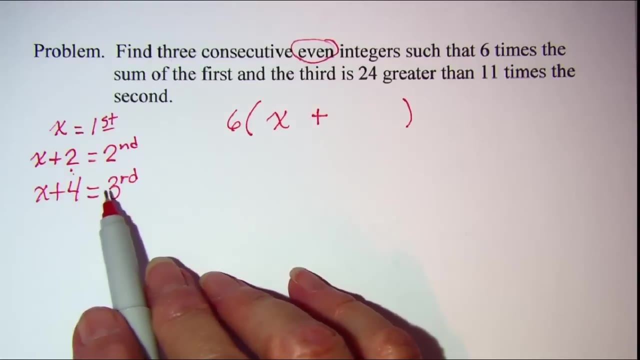 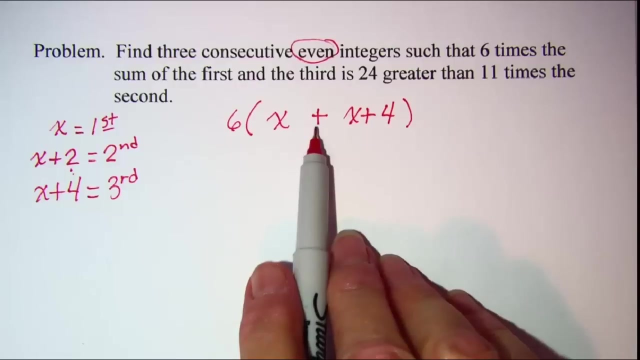 The first is my first integer, so I'll just write x here, and the third, Now my third integer. I need x plus 4 as the expression representing my third integer, so x plus 4 goes in this spot. So this is the sum of the first integer. 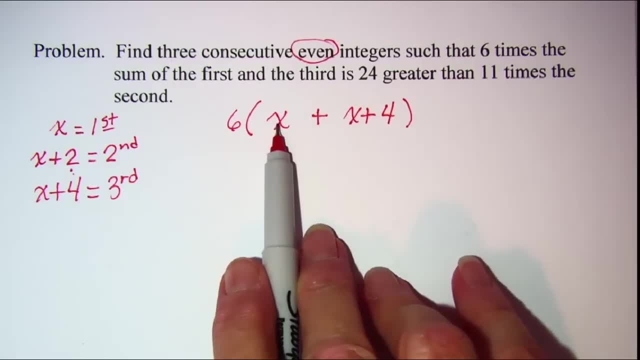 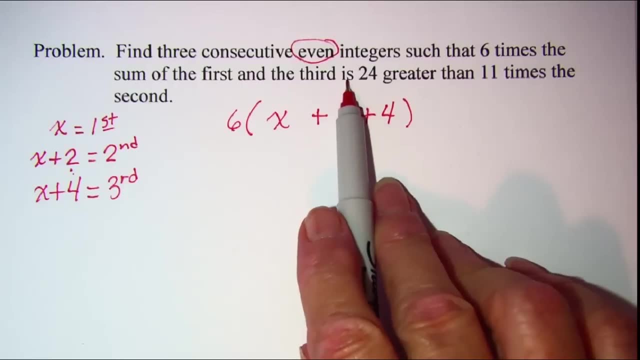 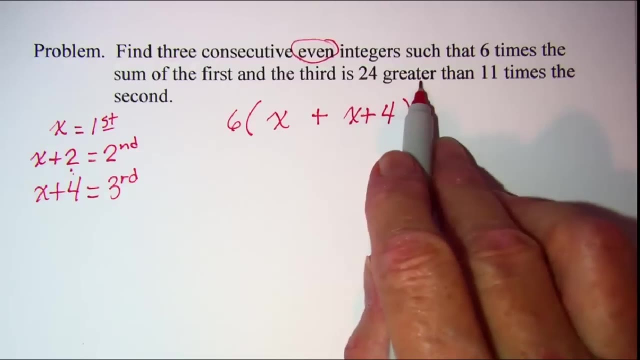 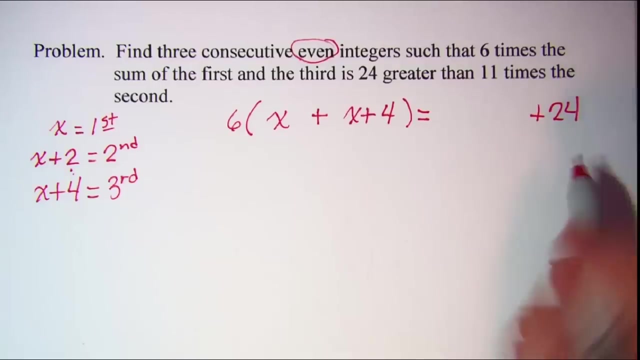 So I'll just write x and the third integer and the third integer. Now let's continue. translating Is: so, that's our verb. so that's where the equals goes. 24 greater than so, I have 24 added on to. 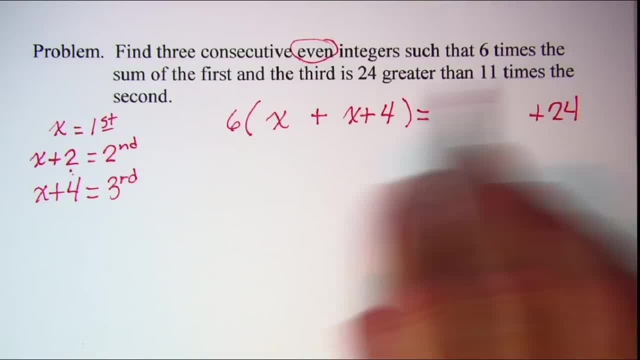 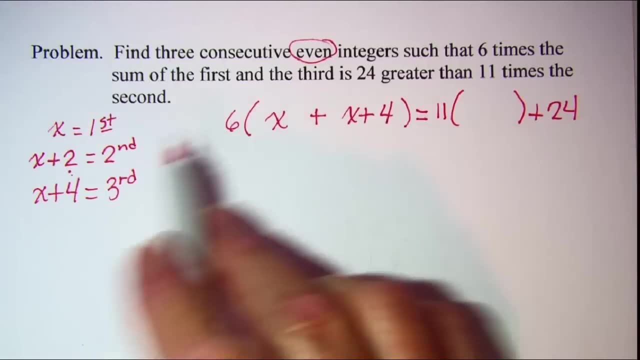 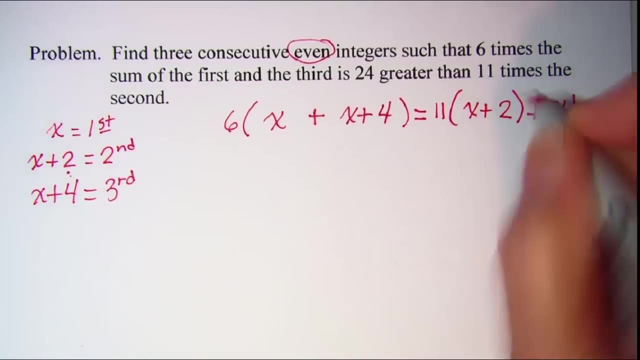 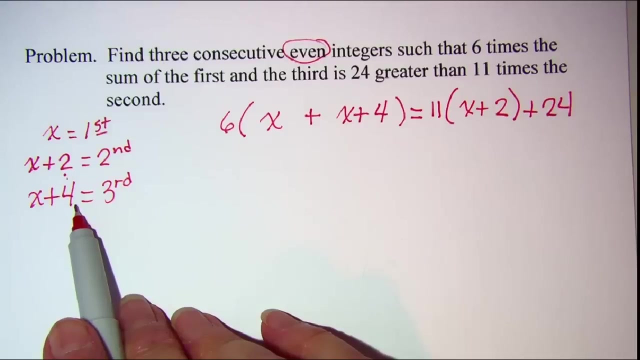 the first and second integer 11 times the second. So I need 11 times, and then in this space I'm going to put the expression for the second integer, which is x plus 2.. So, basically, once you set out these expressions as what you're going to use for your first second, 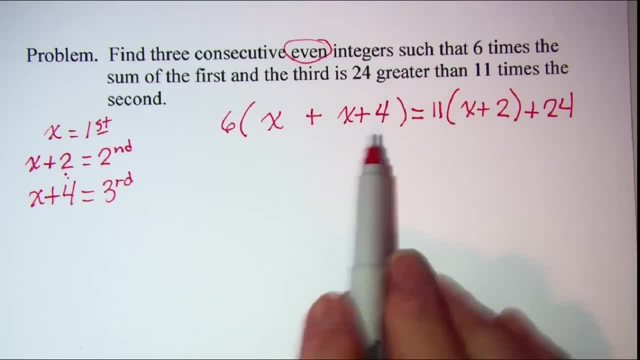 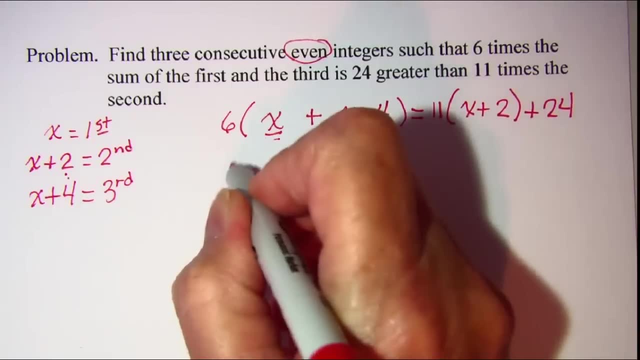 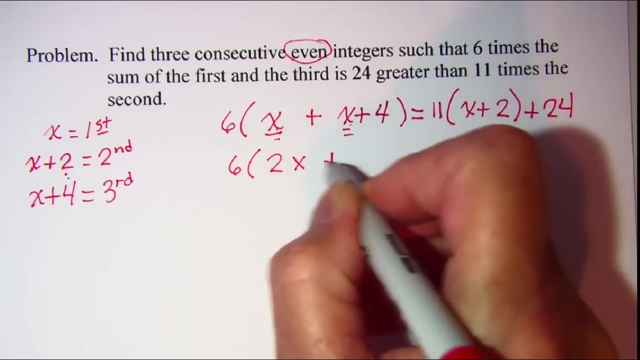 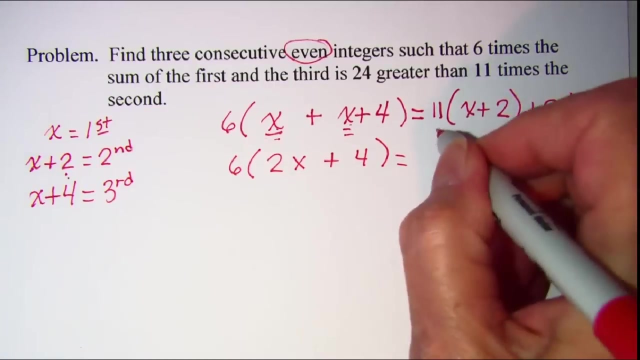 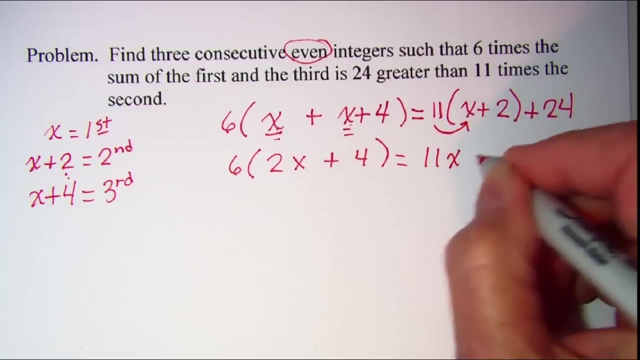 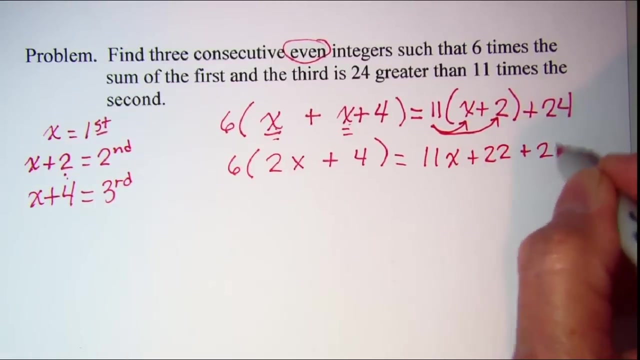 third integers from English into algebra. Let's combine terms here, so I have 6 times the quantity x plus x is 2x plus 4, and then I can distribute this 11 through the binomial: 11 times x is 11x and 11 times 2 is 22.. I just copied the 24 there. 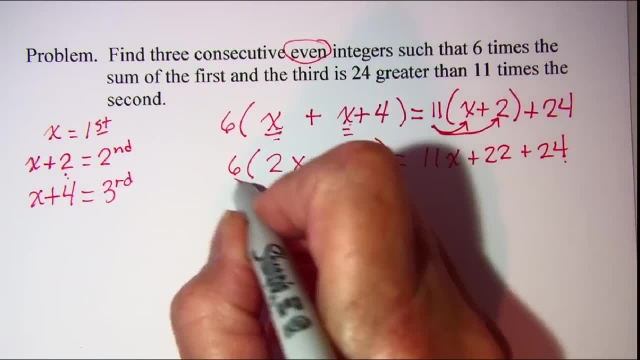 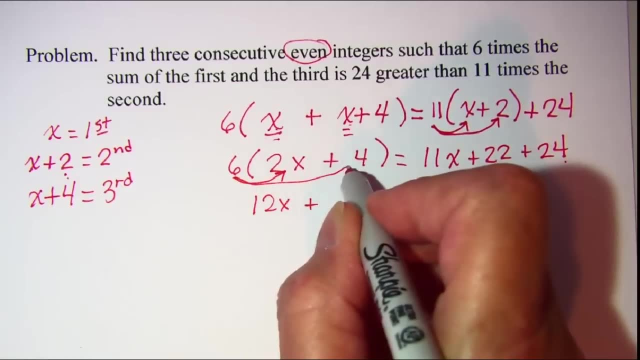 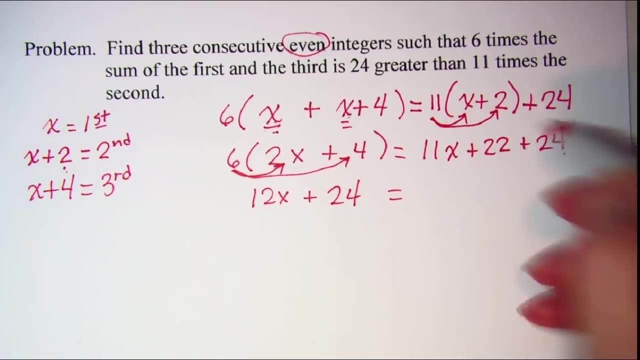 Let's distribute this: 6 through the binomial 6 times 2x is 12x, and 6 times 4 is 24.. On the right side, let's combine these like terms, so I have 11x plus 46.. We'll. 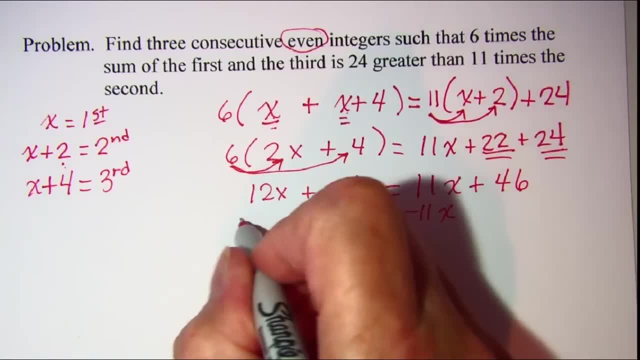 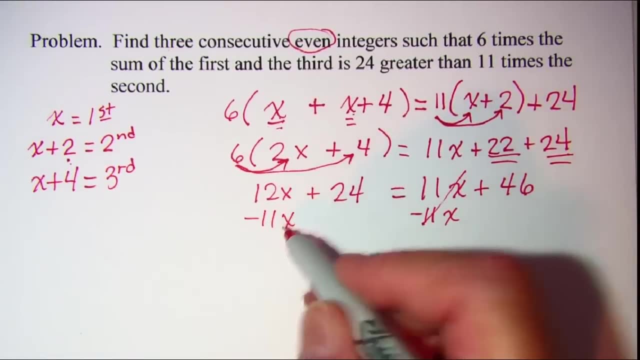 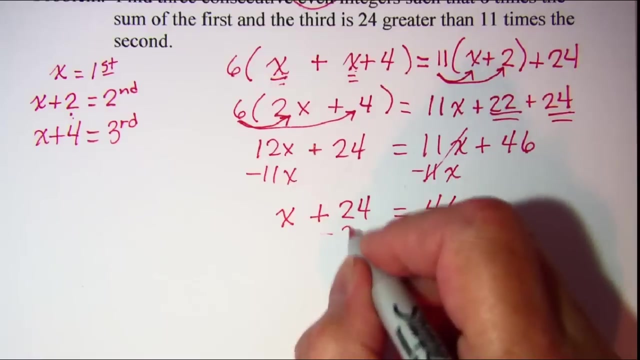 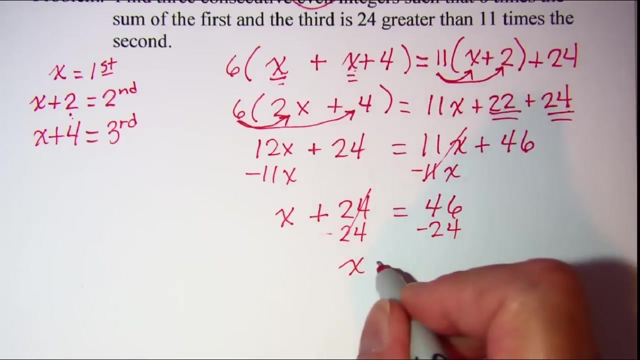 subtract 11x from both sides so that I can put my x's on the left. So cancel here. 12x minus 11x is 1x and just copy and just copy over. here is 46.. Subtract 24 from both sides and x equals 22.. Now